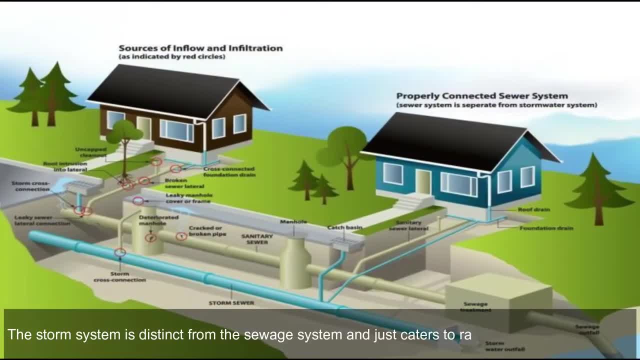 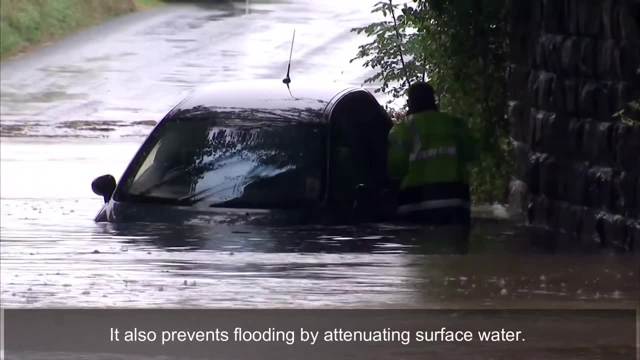 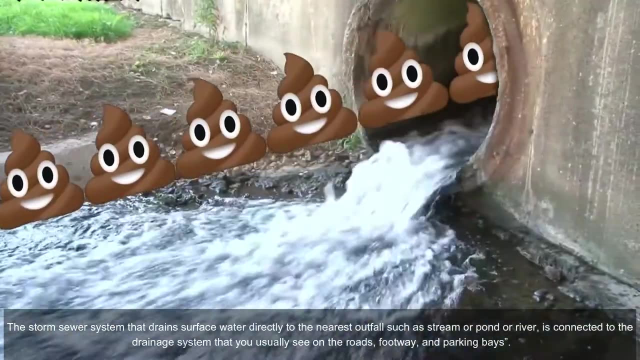 Does storm drains connect to the sewage system? The storm system is distinct from the sewage system and just caters to rainwater and groundwater. It also prevents flooding by attenuating surface water. The storm sewer system That drains surface water directly to the nearest outfall, such as stream or pond or river, is connected to the drainage system that you usually see on the roads, footway and parking bays. 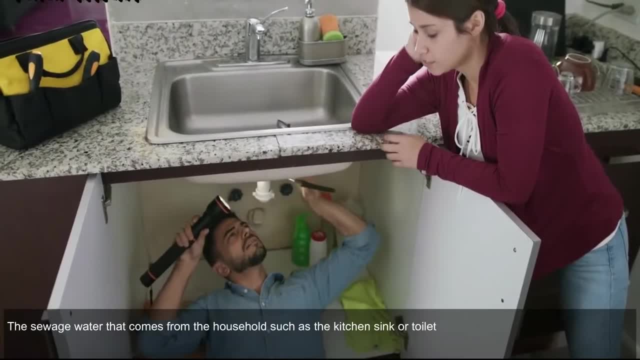 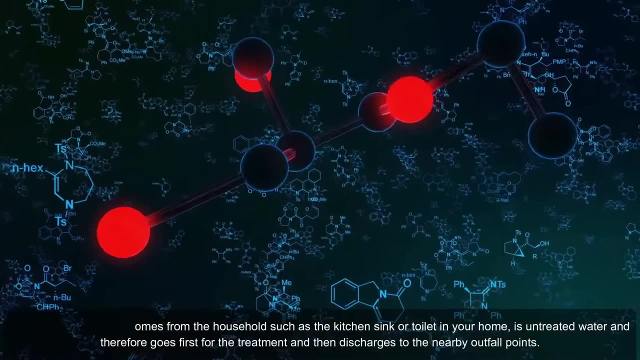 Do storm drains lead to the sea or ocean? The sewage water that comes from the household, such as the kitchen sink or toilet in your home, is untreated water and therefore goes first for the treatment and then discharges to the nearby outfall points. 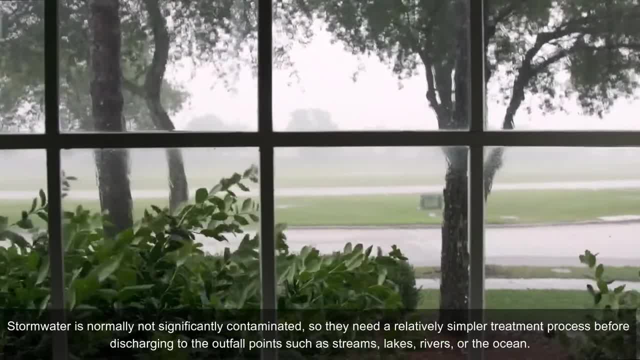 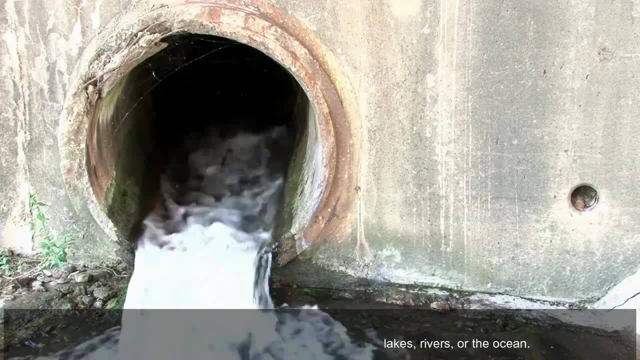 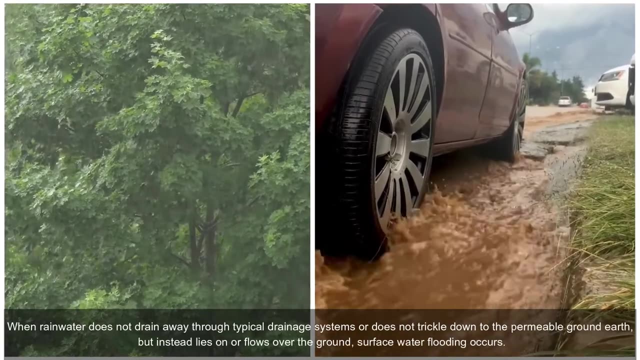 Stormwater is normally not significantly contaminated, so they need a relatively simpler treatment Before discharging to the outfall points such as streams, lakes, rivers or the ocean. What is Surface Water Flooding? When rainwater does not drain away through typical drainage systems or does not trickle down to the permeable ground earth, but instead lies on or flows over the ground, surface water flooding occurs. 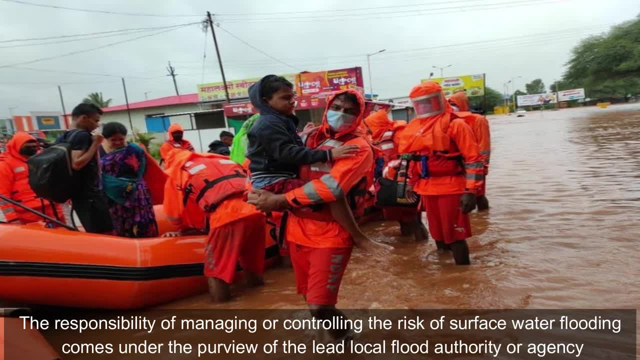 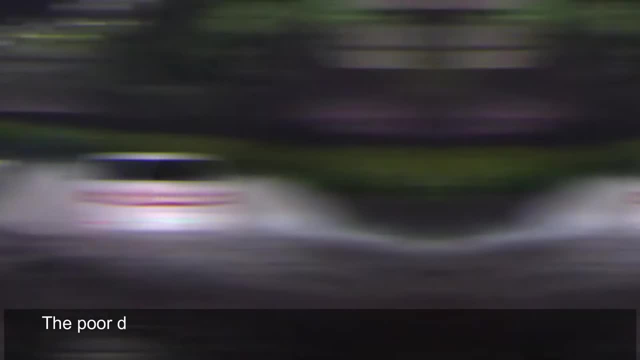 The responsibility of managing or controlling the risk of surface water flooding comes under the purview of the lead local flood authority or agency. What is a Poor Drainage System? The poor drainage system. drainage system can cause flooding, resulting in property loss and possibly causing people. 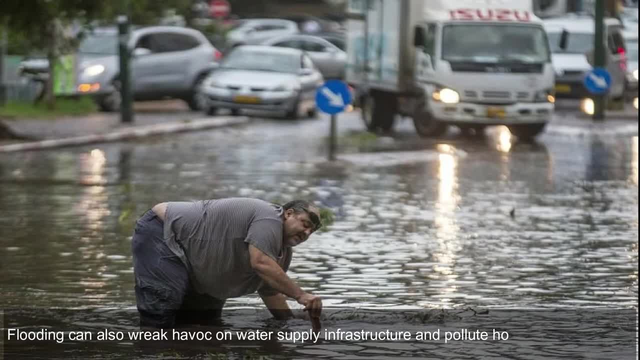 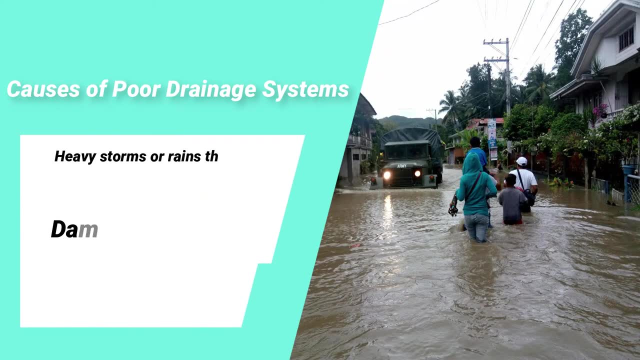 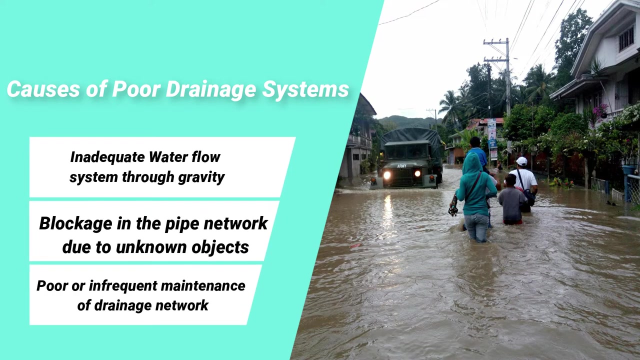 to relocate to avoid the flood waters. flooding can also wreak havoc on water supply infrastructure and pollute home water supplies. following are some well-known common causes of poor drainage systems: heavy storms or rains than the design. pipe network capacity, damaged pipes, incorrect pipe installation, inadequate water flow system through gravity blockage in the pipe network due to unknown. 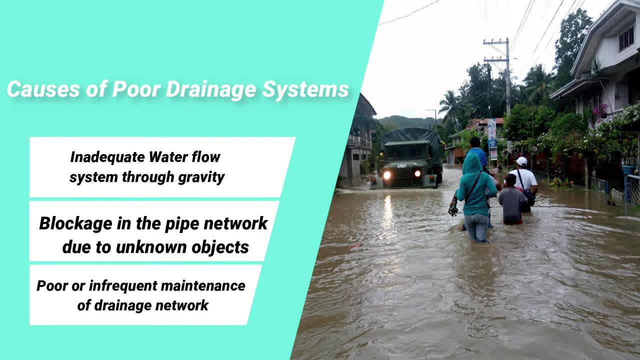 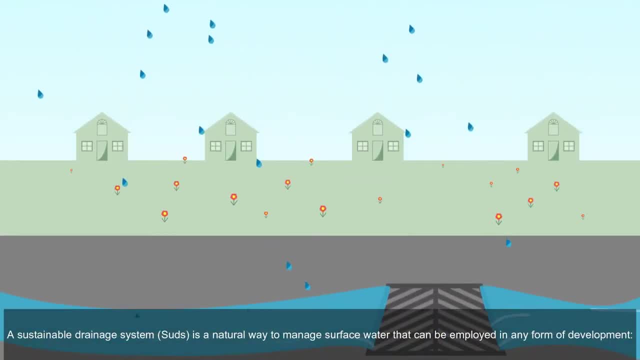 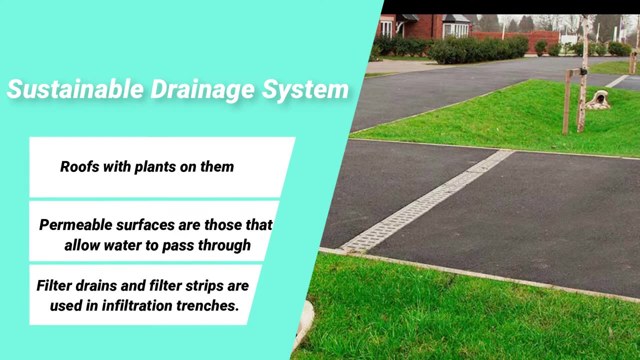 objects: poor or infrequent maintenance of drainage network. how to prevent surface water flooding. a sustainable drainage system- suds- is a natural way to manage surface water that can be employed in any form of development roofs with plants on them. permeable surfaces are those that allow water. 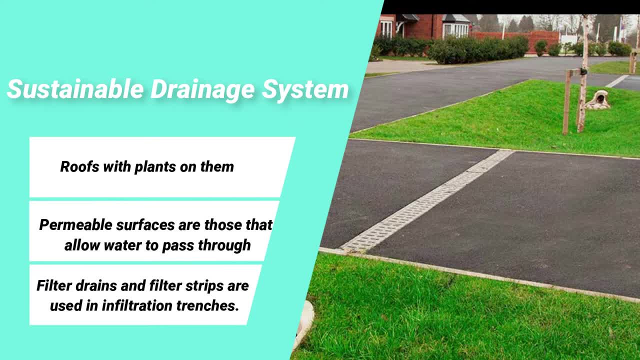 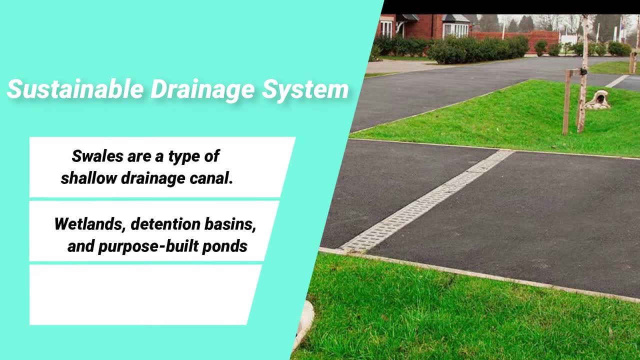 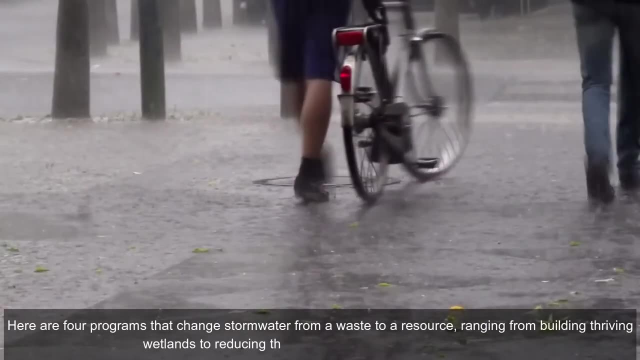 to pass through. filter drains and filter strips are used in infiltration trenches, so are a type of shallow drainage canal, wetlands, detention basins and purpose-built ponds. what are the innovative storm water drainage solutions? here are four programs that change storm water from a waste to a resource, ranging from building thriving wetlands to reducing the 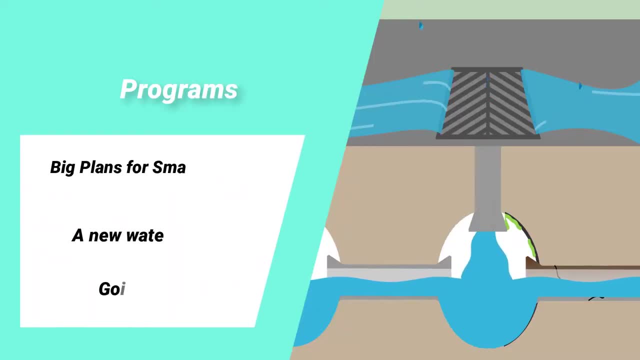 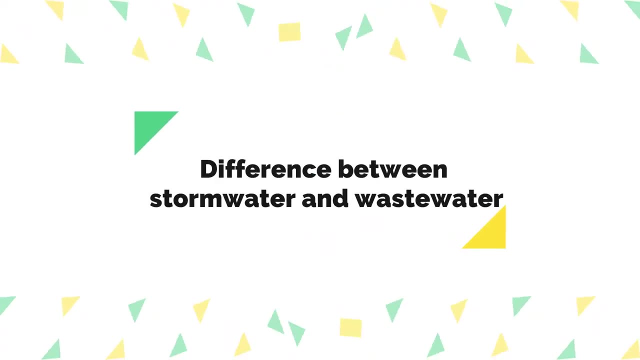 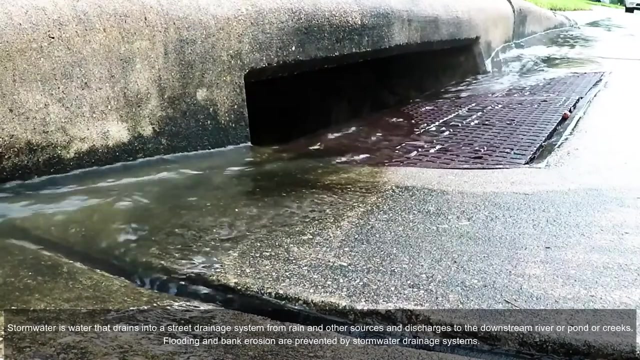 demand for potable water supplies, big plans for small creek, a new water sources, going green. difference between storm water and waste water: storm water is water that drains into a street drainage system from rain and other sources and discharges to the downstream river or pond or creeks. flooding and bank erosion are prevented by storm water drainage systems. 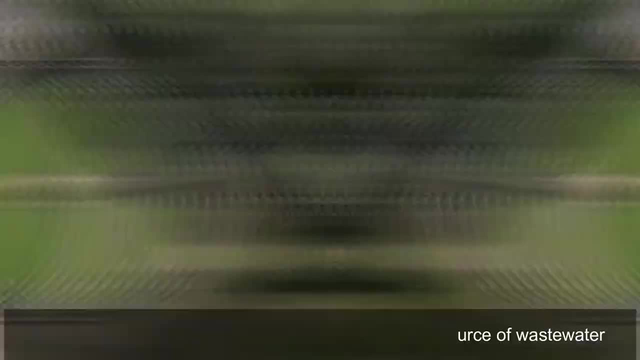 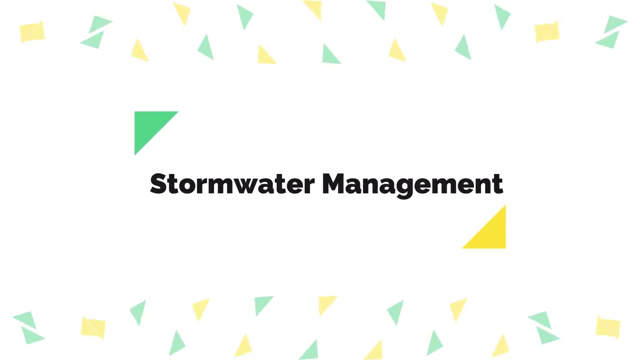 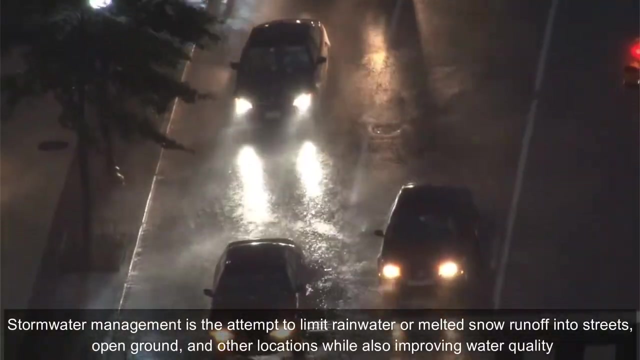 water from households and businesses is the main source of waste water. before waste water is discharged to the nearby streams or creeks, it is very important to treat them storm water management. storm water management is the attempt to limit rainwater or melted snow run off into streets open. 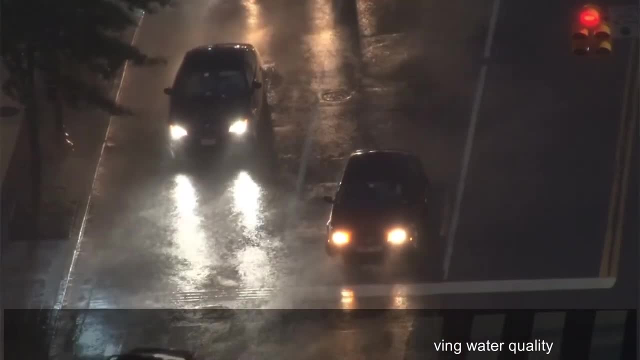 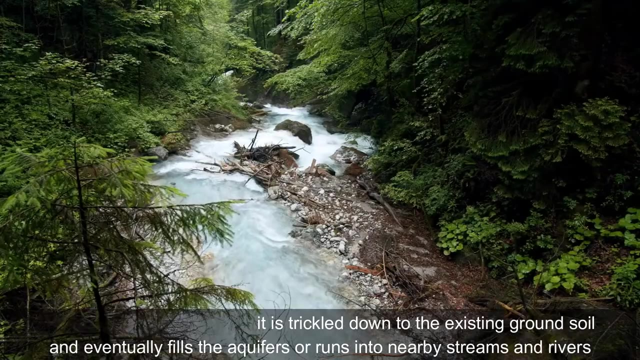 ground and other locations that out of the system that allow water to flow into streams or creeks, while also improving water quality. Storm water is filtered when it is trickled down to the existing ground soil and eventually fills the aquifers or runs into nearby streams and rivers. 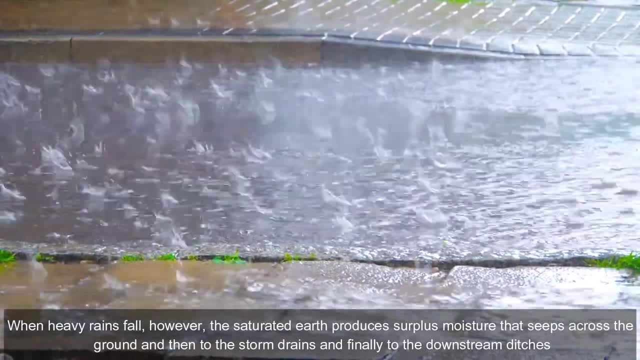 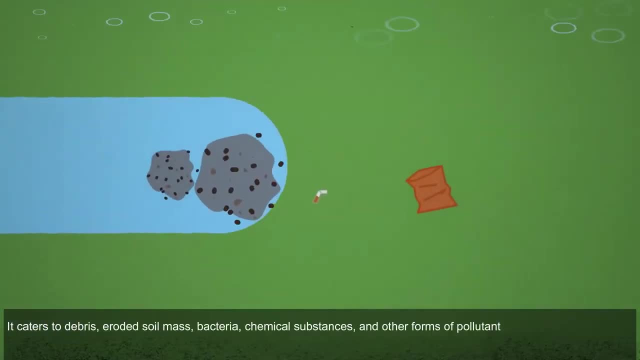 When heavy rains fall, however, the saturated earth produces surplus moisture that seeps across the ground and then to the storm drains and finally to the downstream ditches. It caters to debris, eroded soil, mass, bacteria, chemical substances and other forms of pollutants. 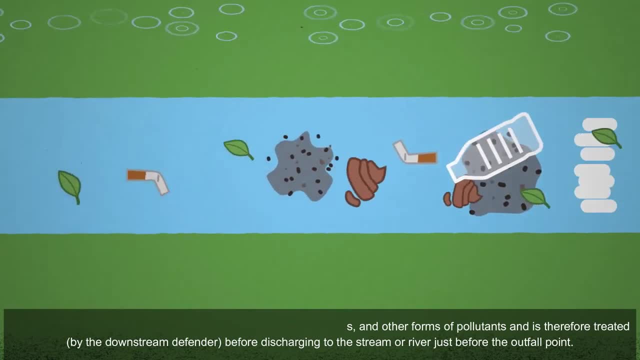 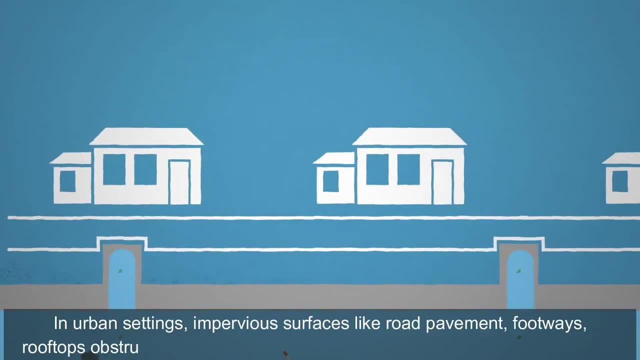 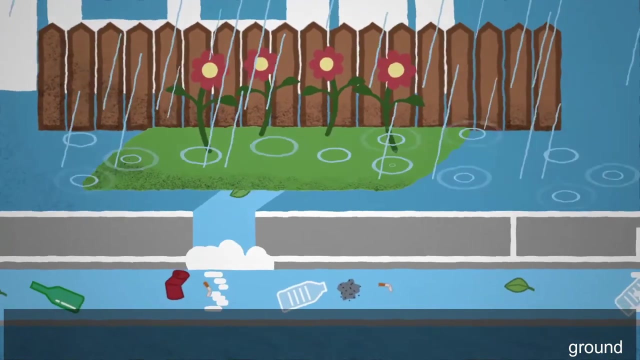 and is therefore treated by the downstream defender before discharging to the stream or river just before the outfall point. How does storm water management help In urban settings? impervious surfaces like road, pavement, footways, rooftops obstruct the rainwater from naturally soaking into the existing ground. 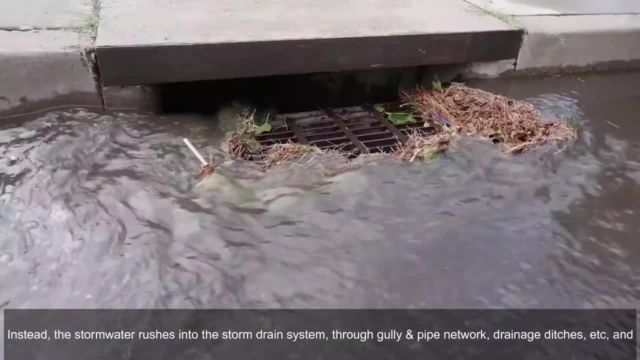 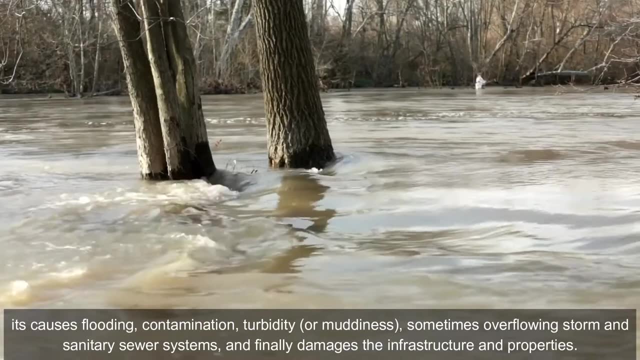 Instead, the storm water rushes into the storm drain system through gully and pipe network, drainage ditches etc. and its causes flooding, contamination, turbidity or muddiness, sometimes overflowing, storm and sand. The storm water occurs in the storm drain system in an area of the gorge in its center. 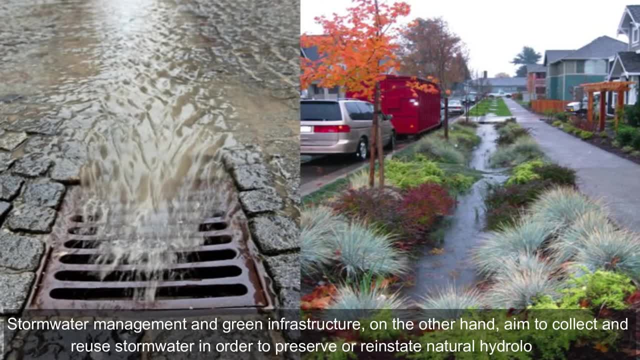 of the gorge or in a floodplain, and is boleh to be constrained by rainwater. Once it comes to storm management, storm water is a new form of sustainability. Storm water is not only used by a system of waterways and rivers, but also for the use. 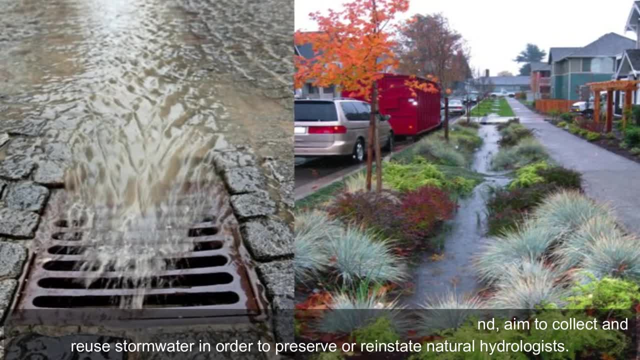 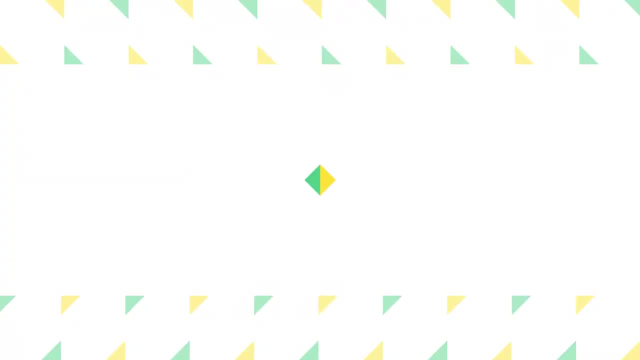 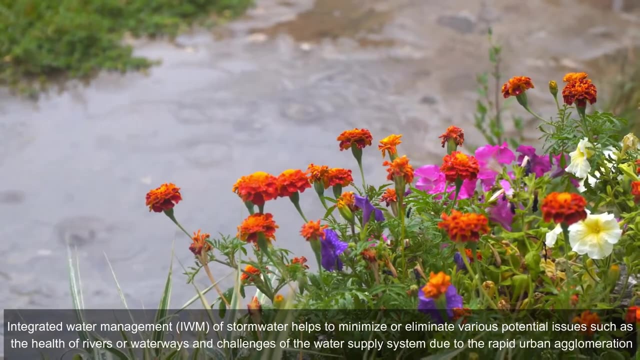 of drinking water and use to help with the плonage of an overhead path and into or near an overflowing gorge. Storm water management is primarily concerned with retaining storm water and eliminating pollutants. Integrated water management: Integrated water management, together with storm water, helps to minimize or eliminate.